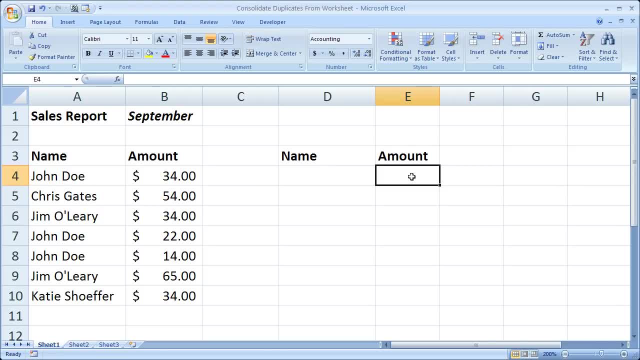 So that's the goal of this tutorial, And I'm going to show you how to do that with the consolidate command. This is a great feature of Excel 2007.. Before I do that, though, make sure you have copied the headings to a new location, So you can't bring the headings with you. So new headings: Select where you want the consolidated data to go. You have to do that before you consolidate. Then go to the data tab. 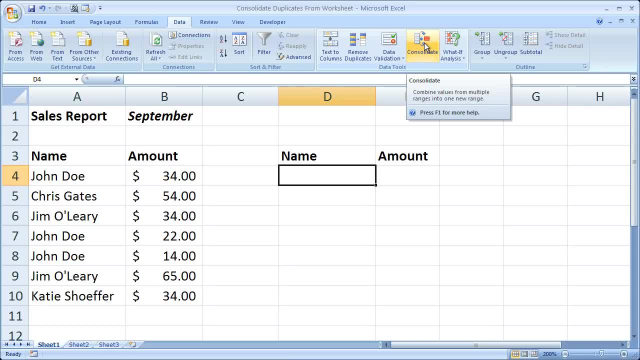 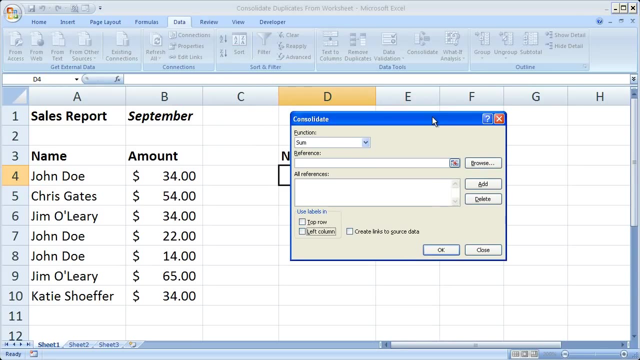 And select consolidate, And if your Excel window is a little bit smaller than mine, this may be a small bar, But it's in the data tools window, So go ahead and click consolidate And then a window like this is going to open up. So what we have here is the function that we would like to perform when we consolidate, And most times it's the sum function. You want to add everything together, And in this case we want to add everything together. We want to add John Doe's expenses for the month. 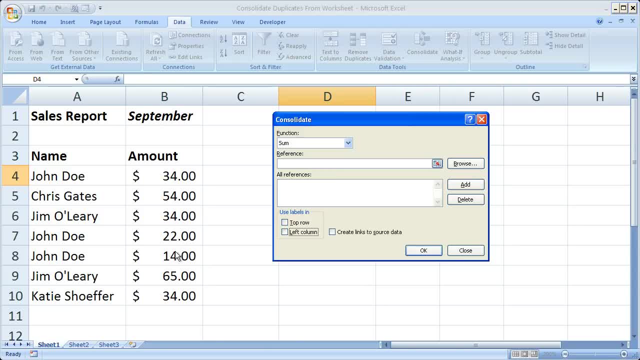 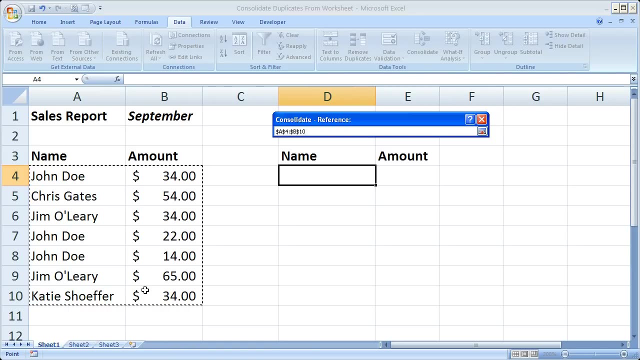 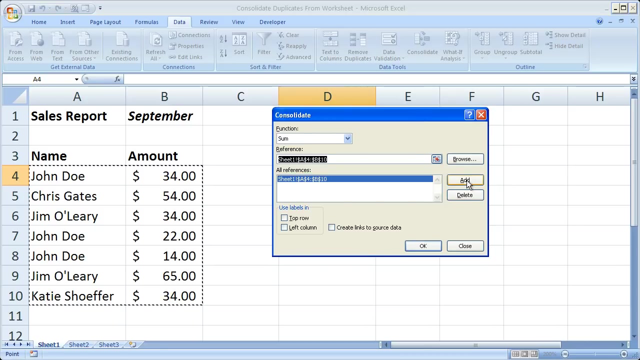 Together to create one number. The next thing is the actual reference, So where the data is that we would like to consolidate. So I'm going to go ahead and select that right now. When you've selected that, go ahead and click this button again. The next thing is to hit add, And the reason it says all references here are because you can actually use this feature to consolidate range. 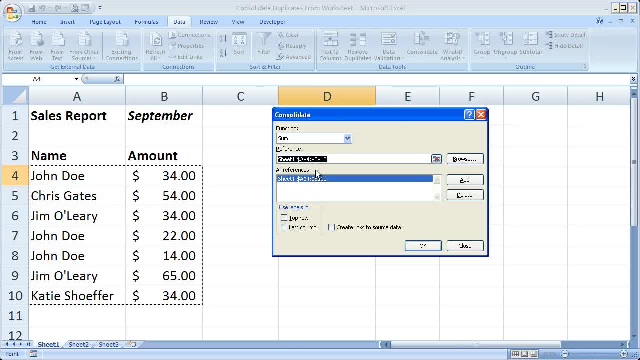 So you can add ranges of data from multiple worksheets at once, As well as multiple different workbooks at once, But today we're just going to use the very simple feature to add these things together. So now we've got the function that we'd like to perform: Sum The values that are exactly the same from the same person, And then we have the reference. Now the most important thing here is use labels. in This little box right here, You can select top row. 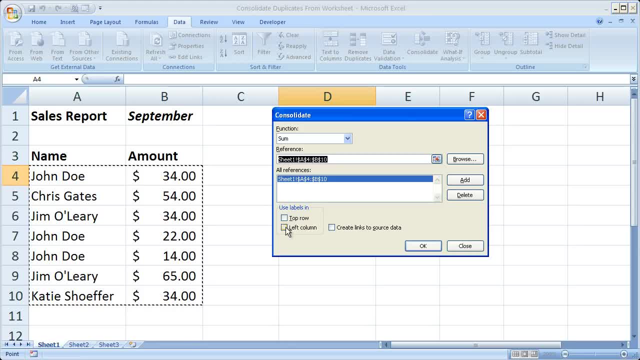 Or left column, And the labels are what it's going to use to actually figure out where the multiple values are, So where John Doe is throughout the list. So are the names for the customer's in the top row Or are the customer names in the left column?